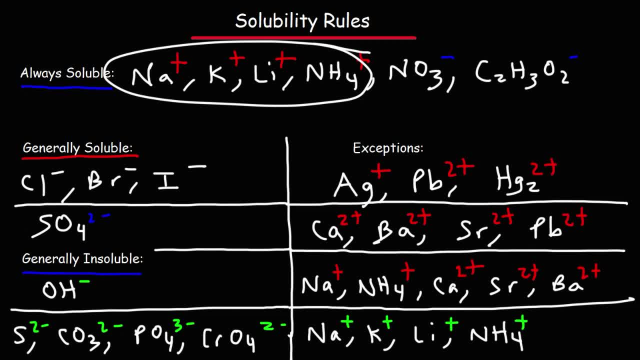 And the group 2, sodium, potassium and lithium, And, of course, with ammonium. So those are the general solubility rules that you need to be familiar with. If you know this, this is good enough to determine if a compound is soluble or insoluble. 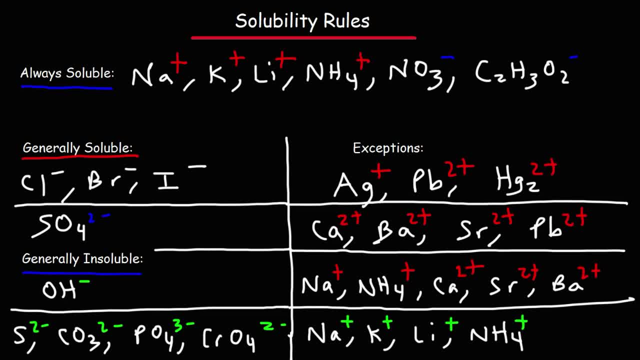 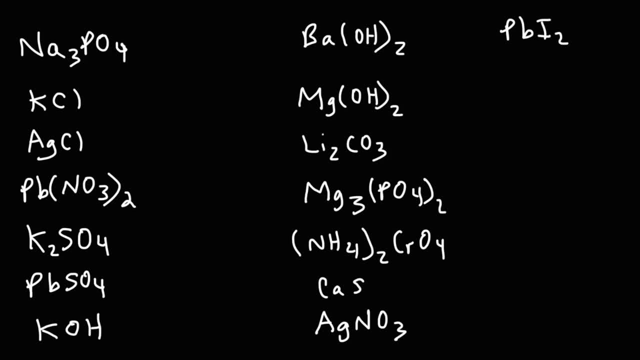 Now let's put this information to work. Let's put it into practice. Let's work on some example problems. Let's start with this one: Sodium phosphate. Is it soluble or insoluble? It's soluble on the solubility rules anytime you see a group 1 metal ion like sodium, potassium or lithium. 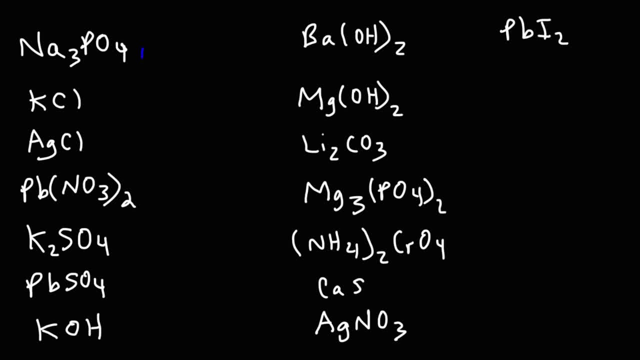 it's going to be soluble, And so we're going to represent this using the phase aq, aqueous, which means that it dissolves in water. Now, what about potassium chloride? Well, potassium is a group 1 metal, so that also will dissolve in water. Now, silver chloride chlorides are generally 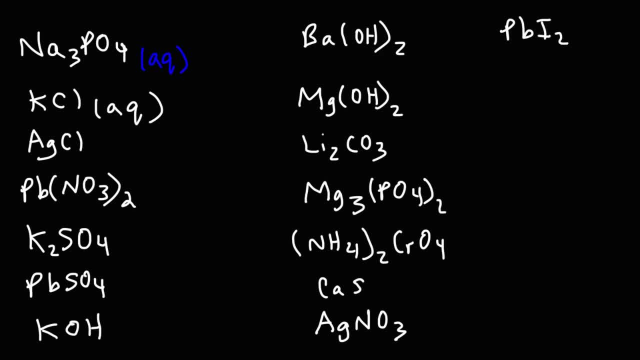 soluble, with the exceptions of silver, lead and mercury. So, because that is an exception to being generally soluble, this is going to be insoluble and we're going to write s because if you were to mix sodium chloride in water, it's going to remain as solid. It's not. 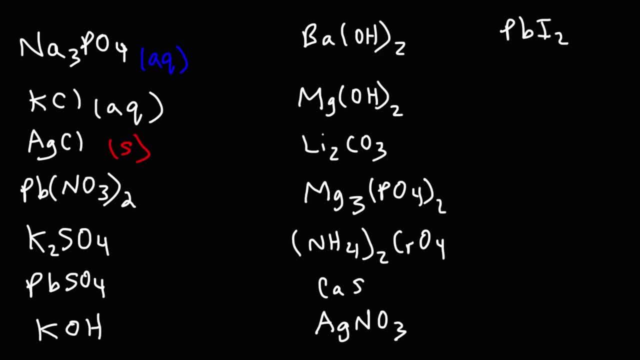 going to dissolve into the aqueous phase. Now what about lead nitrate? Nitrates are always soluble, so we're going to put that in the aqueous phase. Next, potassium sulfate. Potassium is a group 1 aqueous, one metal cation, and so that is going to dissolve in water. that's soluble, so we're going to write. 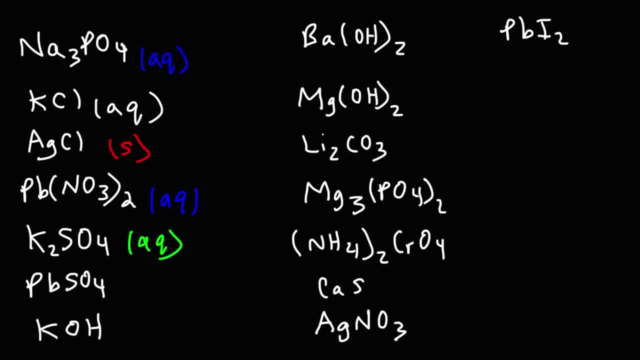 aqueous, let's use sulfate. sulfates are generally soluble, but lead is an exception, so this is going to be insoluble in water. next we have potassium hydroxide, potassium being a group one metal that's always going to be soluble, so we're going to write aqueous for that. 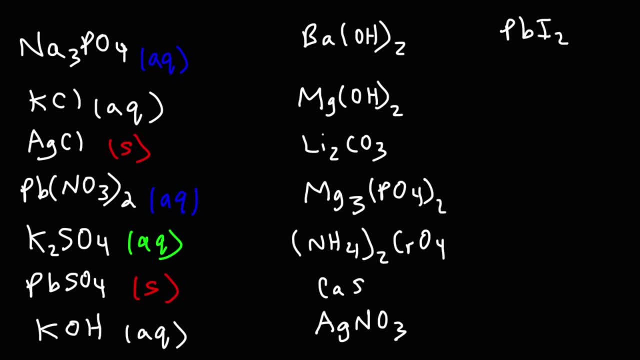 now it might be a good idea to pause the video. take out a sheet of paper and try the remaining examples yourself. determine if these compounds are soluble and insoluble using the solubility rules that we discussed earlier in this video. so feel free to take a minute to try these problems.